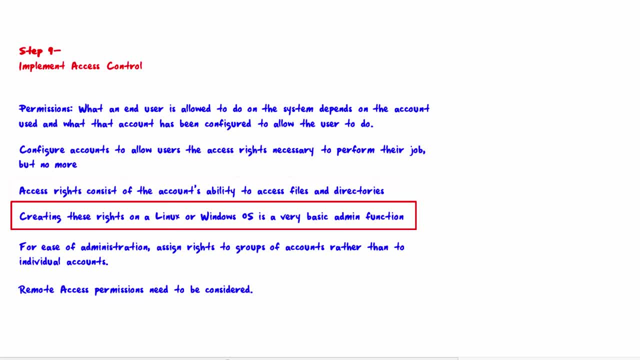 Creating these rights on a Linux or Windows OS is a very basic admin function, so we won't go into the specifics here. For ease of administration, assign rights to groups of accounts rather than to individual accounts. You should create groups of employees with a similar job function and then assign specific. 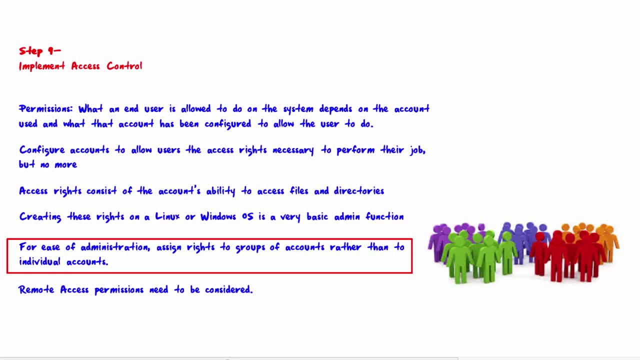 rights to the group. For example, all junior accountants will get a specific set of permissions, while all senior accountants will get a different and probably more permissive set of permissions. All admin assistants will get a specific set of permissions applicable to their job duties, etc. 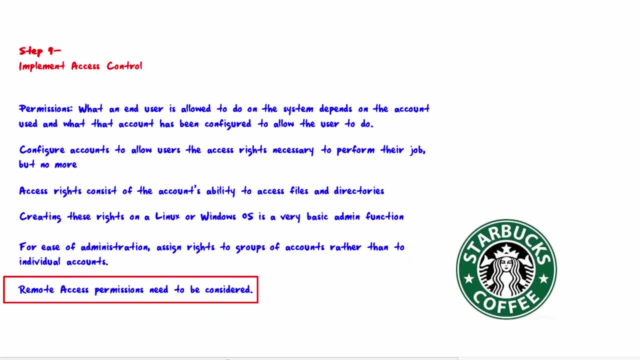 Remote access permissions need to be considered carefully. That is, if Huckleberry is allowed a specific set of permissions if he is sitting in the home office, is he allowed those very same permissions if he is sitting at home or if he's sitting in a hotel room or starbucks? 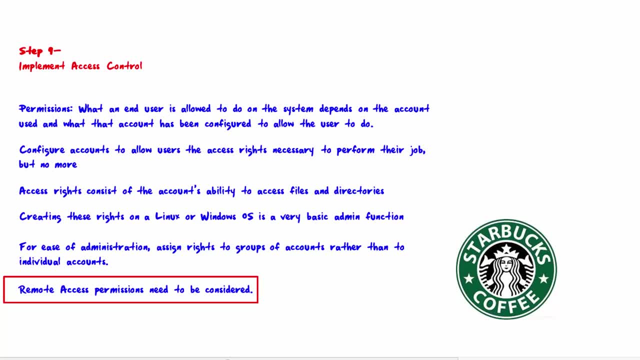 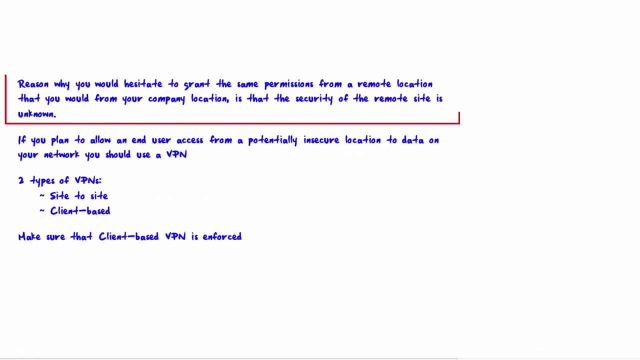 for ease of use, many companies will allow huckleberry to have the same or similar permissions wherever they're physically located, but you should carefully consider the security applications prior to granting such permission. the reason why you would hesitate to grant the same permissions from a remote location than you would from your company location. 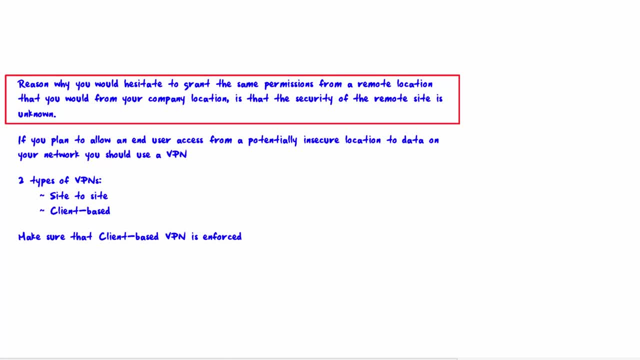 is that the security of the remote site is unknown. if you plan to allow an end user access from a potentially insecure location to data on your network, you should use a vpn. a vpn provides secure communication over an insecure public network. so what's going to happen is the data that goes back and forth will be encrypted. 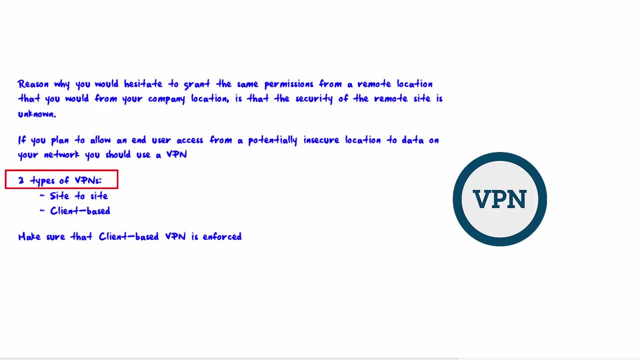 now there are two types of vpns: site to site vpns and client-based vpns. what we're talking about here is client-based vpns. here, a piece of software is installed on the end user's laptop. this allows the remote user to a establish a VPN from his laptop to the security appliance that sits on your home network.